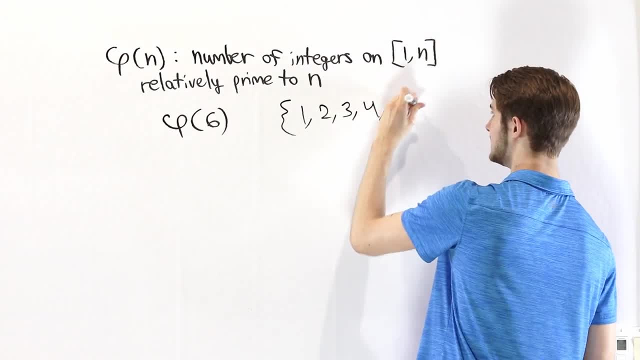 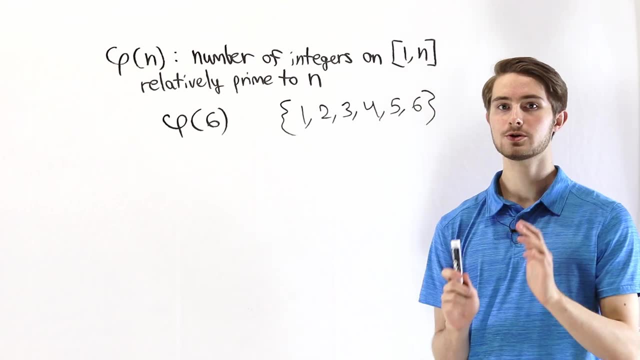 1,, 2,, 3,, 4,, 5, and 6.. So we want to find the number of integers in this set that have no common factors with 6.. We know that 6 is equal to 2 times 3.. 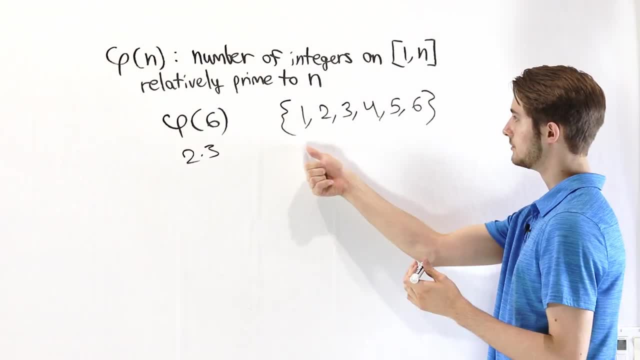 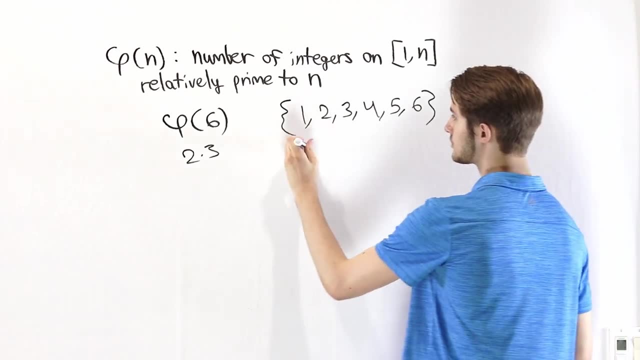 This is the prime factorization And therefore we need to find the numbers that don't have a 2 or a 3 in their prime factorization. That's going to be 1, not 2, because that is a prime factorization. 4 is equal to 2, not 3.. 4 also includes a 2 as well: 9,, 9,, 9,. 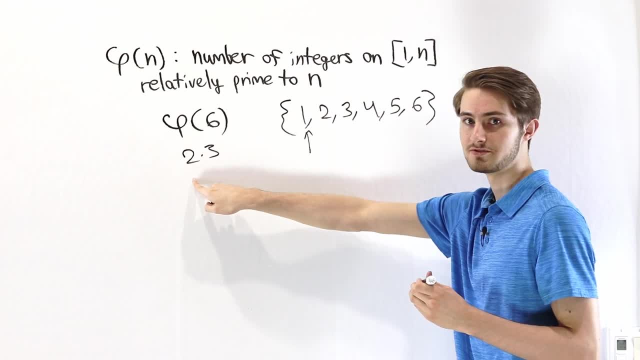 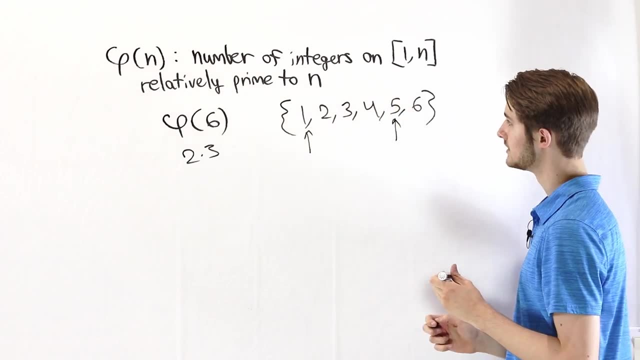 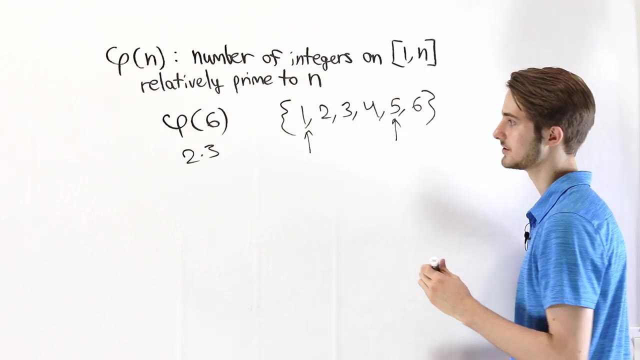 9,, 9,, 9.. So even though 4 doesn't divide 6, it still has a common factor. On the other hand, 5 is definitely a prime factor and then 6 is not. So we see that there are two integers on 1 to 6 that are co-prime to 6, and then 5, 6 is equal to 2.. 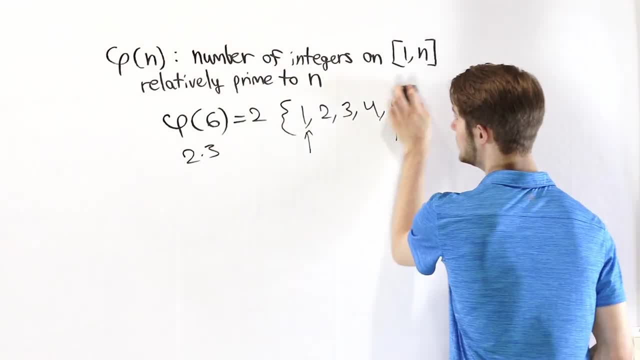 Now we're going to look at some specific examples of the totient function, which are the common, but they have no common factors: 3, 2, 3, 4,, 4, 5, and 6.. when we look at some prime numbers, Let's start off with the simplest case. 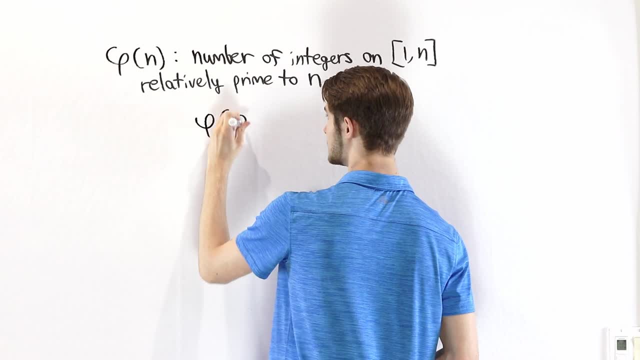 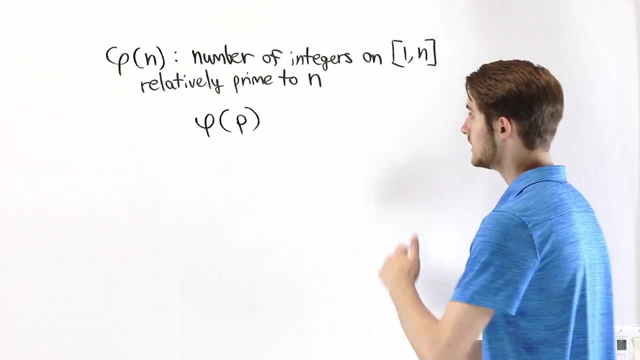 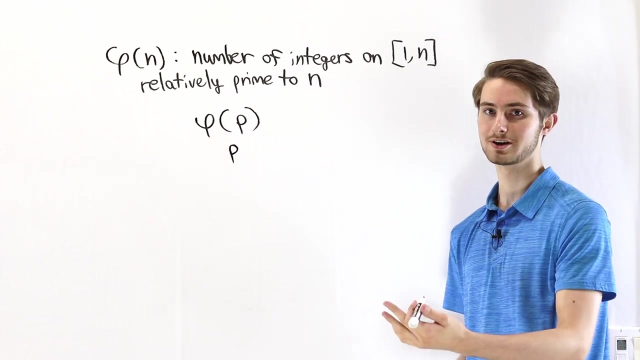 of the Euler's Totient Function. What is the Totient Function of a prime number? So in this case we're saying that p is prime. Well, remember that the prime factorization of a prime number is just p. It is its own only prime factor And as a result of that, 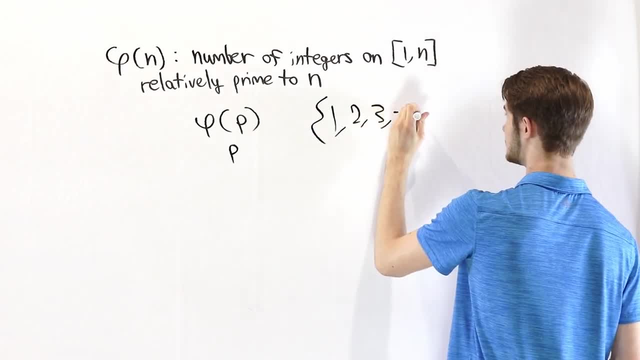 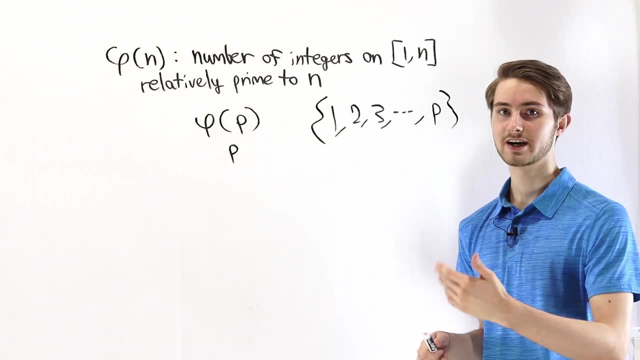 if we look at the interval 1,, 2,, 3, and so on up to p, none of these numbers in here are going to share any factors in common with p, because in order to share a factor with p, they would have to include p in their 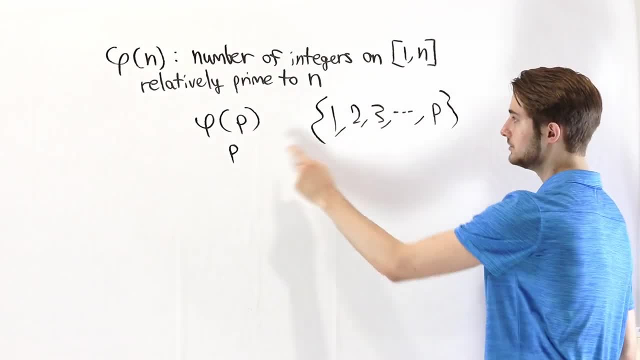 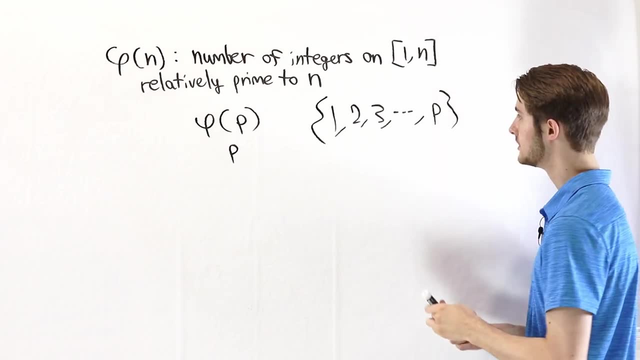 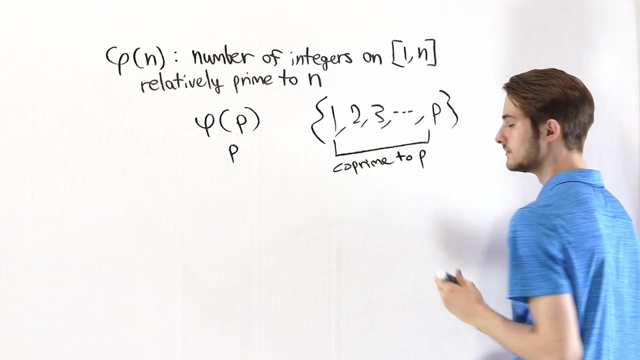 prime factorization. But it's impossible to include p in your prime factorization and still be less than p. You'd have to be at least equal to p, Which means that all of the numbers in here are co-prime to p. Of course, p is not co-prime to p because 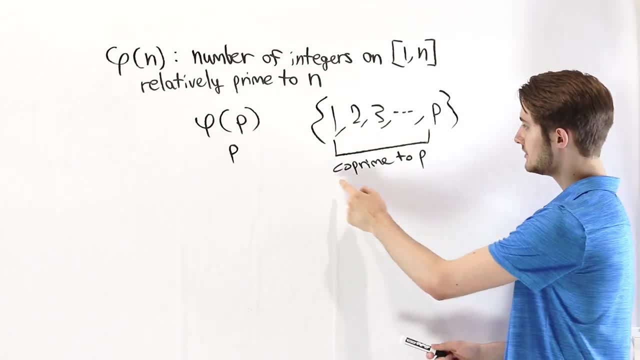 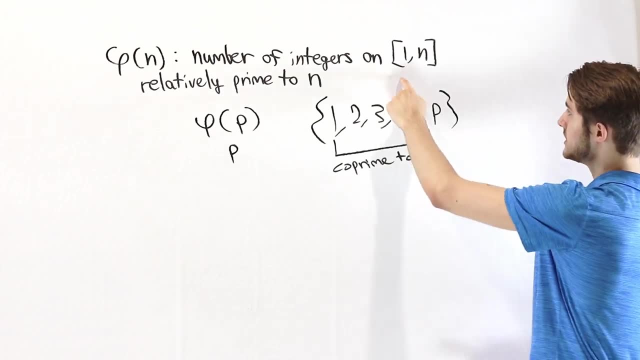 it's equal to itself. Now we want to find the number of integers that are co-prime to p. That's going to be the number of integers in here. Well, that's all the numbers on the interval 1 to p, except for p. 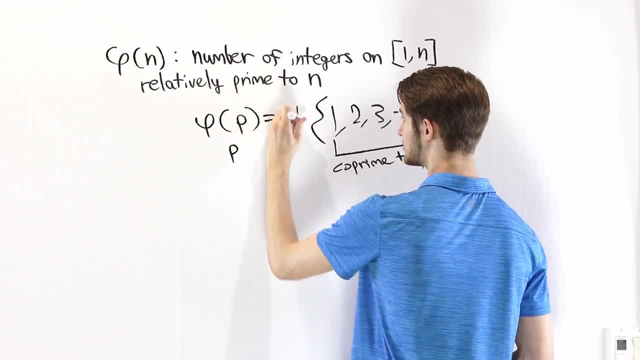 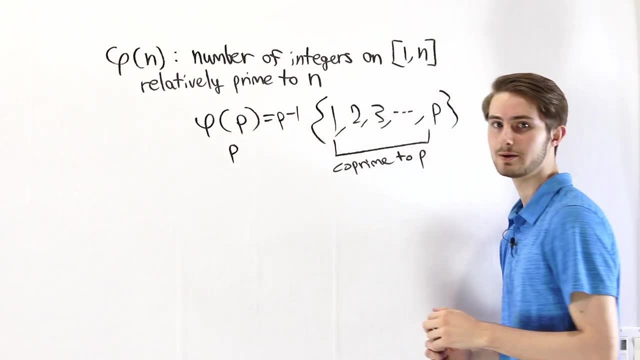 And the number of numbers in that interval is just p minus 1, since we're not including p. So for any prime number, the totient function of that prime number is equal to p minus 1.. For example, the totient function of 13 is equal to. 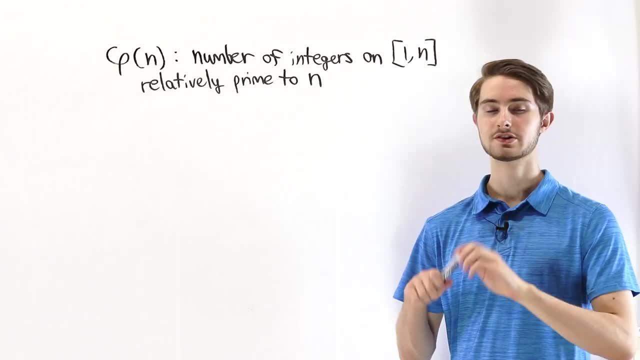 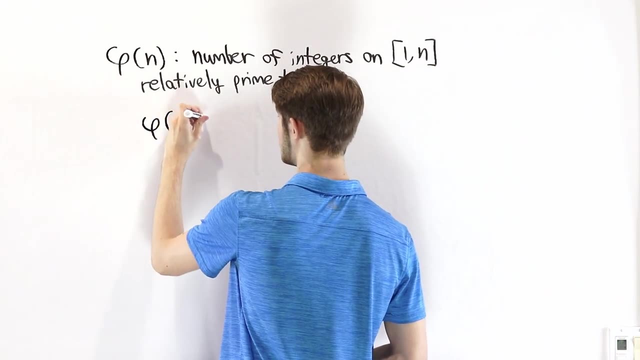 12, since 13 is a prime number. So now we've seen the simple example of phi, of a prime number. Now we're going to look at a slightly more general result, which is the totient function of p to the power of some number. 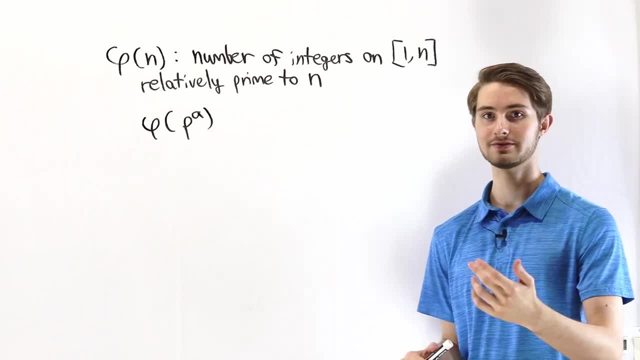 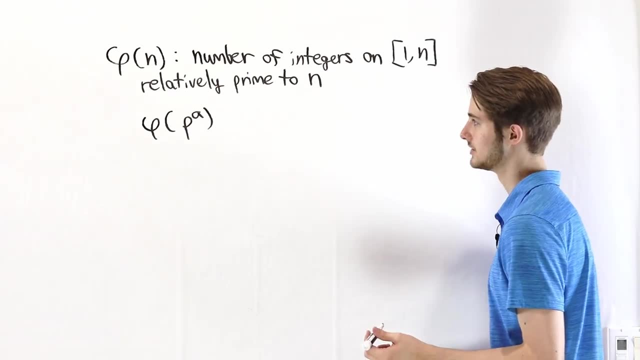 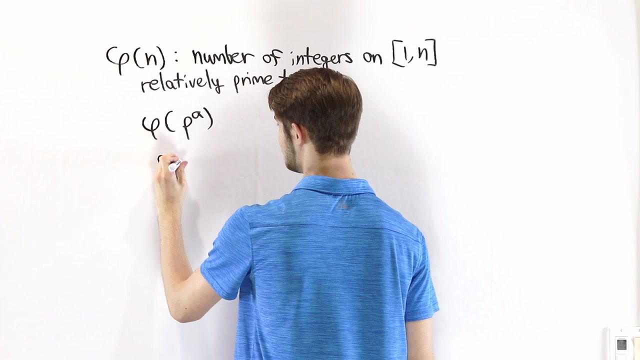 So p is still a prime number, but now we're choosing some positive integer as an exponent. To figure out what this is, we first need to look at the prime factorization. Now, of course, because p is prime, the prime factorization of p to the a is going to look like p times, p times, p times, and so 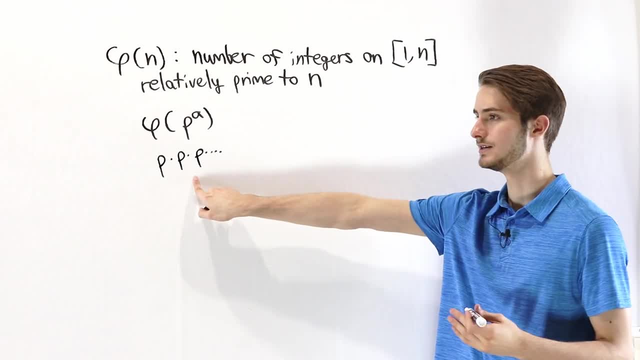 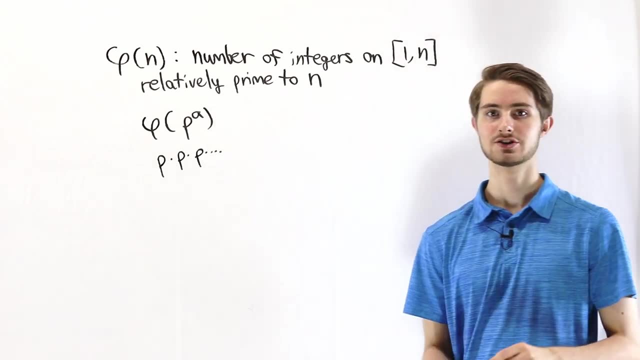 on. So the only prime factor is p. What that means is that all of the numbers that share a factor with p to the a are just all the multiples of p. What are those? Well, that's going to be p 2 times p. 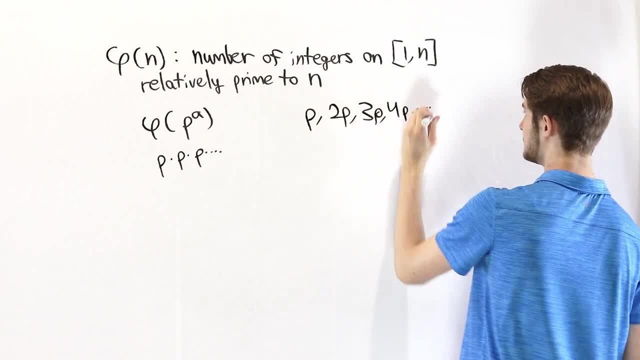 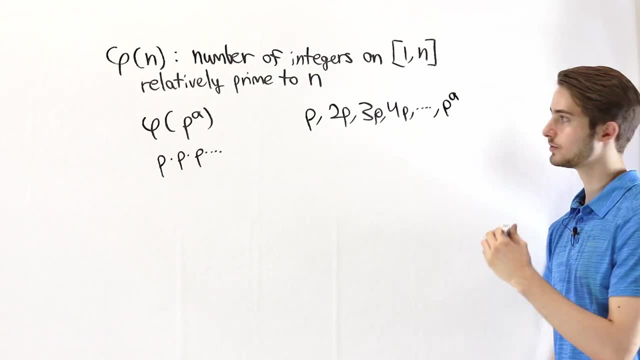 3 times p, 4 times p and so on all the way up to p to the a. This is the last number in our interval And we can also write p to the a as p to the a minus 1 times p. 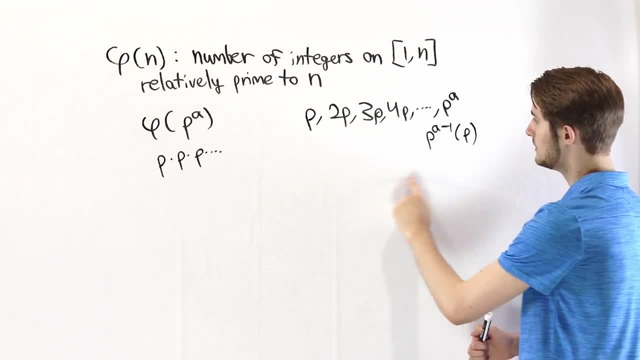 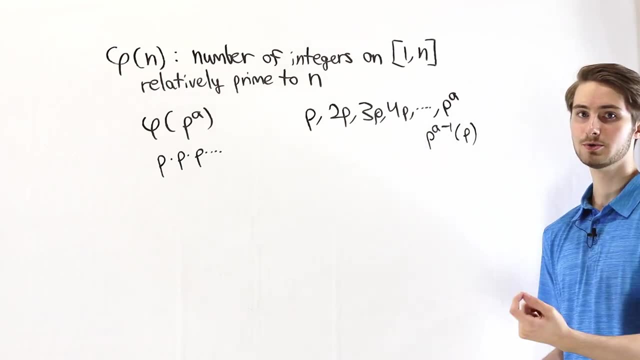 The reason that we do this is because our goal here is to count the number of integers in this set, And we can see that all of these are just multiples of p. So the number of multiples there are is 1,, 2,, 3,, 4,, 5,, 6,, 7,, 8,, 9,, 10,, 11,, 12,, 12,, 13,, 13,, 14,. 15,, 12,, 13,, 14,, 15,, 16,, 16,, 17,, 18,, 19, 20.. So we're going to divide that by 2,, 3,, 4,, 5,, 6, up to p to the a minus 1.. That's how many multiples of p we have. So we're looking at p to the a minus 1 numbers that share a factor with p to the a. But remember that our goal is not to find all of the numbers that share a factor with. 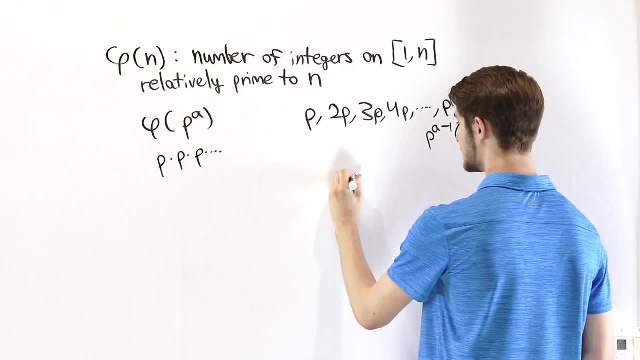 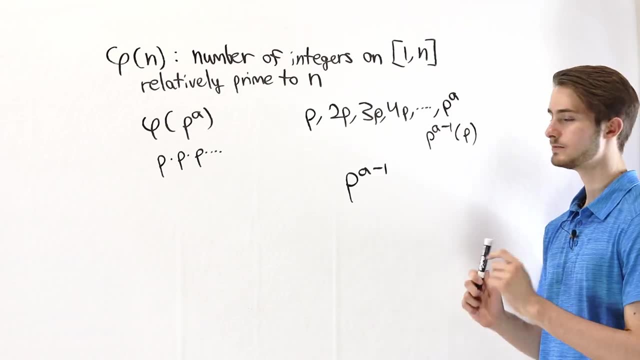 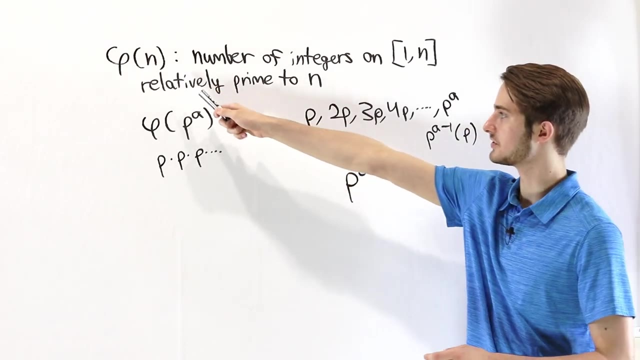 p to the a. Our goal is to find all of the numbers that are relatively prime, In other words, they share no factors with p to the a, And that's going to be all of the numbers that share a factor with p to the a.